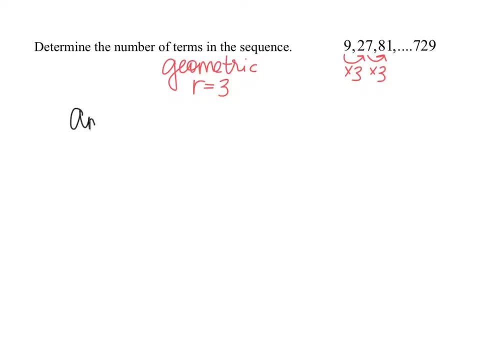 So, with this information, we can go ahead and write a general formula for this sequence of numbers. So, knowing that it's geometric, we have a general formula for any geometric sequence which is a sub 1 is, excuse me, a sub n. 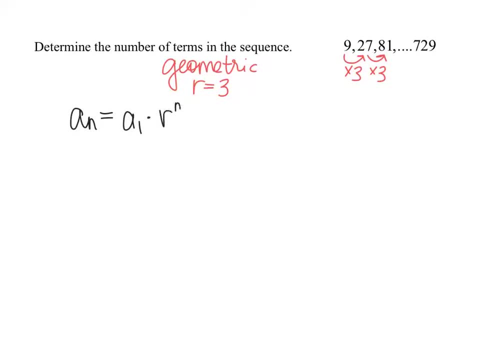 It's equal to a sub 1 times r raised to the n minus 1 power, And we know the first term is 9.. The r value, the common ratio, is 3.. So that would be 9 times 3 raised to the n minus 1 power. 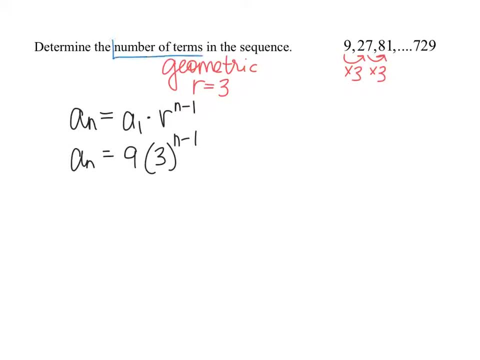 Now, in this case we're trying to find the number of terms in the sequence. So what that really means is we are trying to solve for n. n represents the number of terms, But we are given the last term in the sequence, which is 729.. 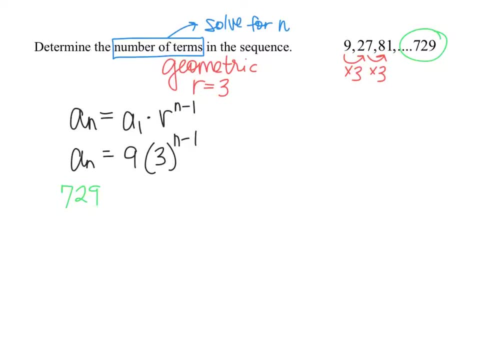 So we can go ahead and substitute 729 in for a sub n, the last term of the sequence, and then just solve for n, And that will tell us which term that is Now. of course we could certainly get out our calculators and continue multiplying by 3 repetitively. 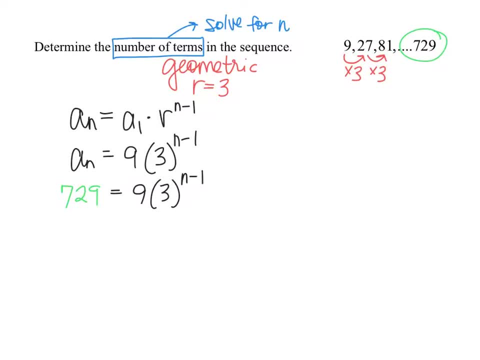 until we eventually land on 729.. But, as my college professor as math would say, that wouldn't be a very elegant solution, So we're trying to be more efficient. So what we have here is an equation we need to solve, And this is actually an exponential equation. 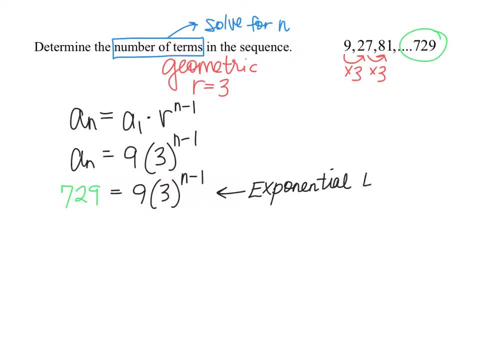 So we want to work to isolate the exponential piece of this equation. So that means the exponential piece. if I highlight that for you, that would be the 3 raised to the n minus 1 power. So therefore we need to divide both sides by 9 so we can isolate the exponential quantity. 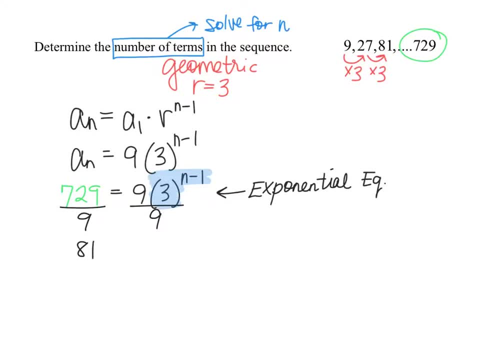 729 divided by 9 will give us 81. So 81 is equal to 3 raised to the n minus 1 power. Now my base on the right-hand side is 3.. So on the left-hand side I can rewrite 81.. 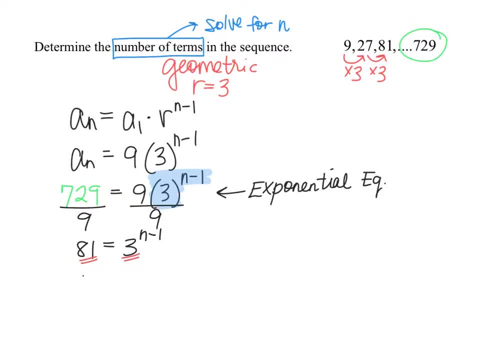 So that is also base 3, because 81 is actually 3 raised to the 4th power. So if I rewrite 81 as 3 to the 4th, that equals 3 raised to the n minus 1 power, And now I have achieved common bases on both sides.